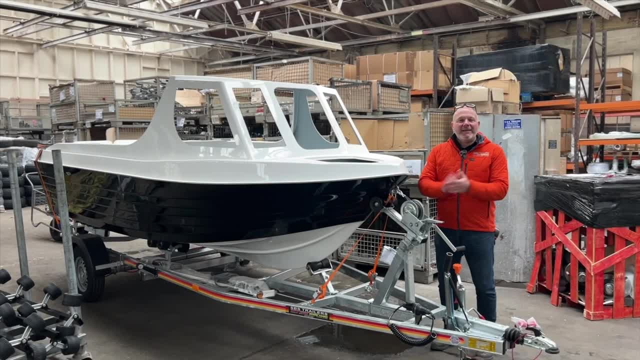 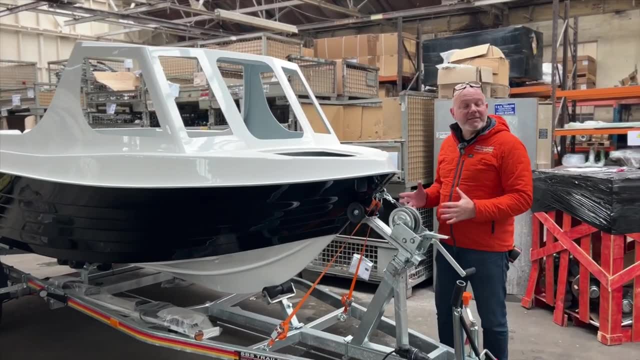 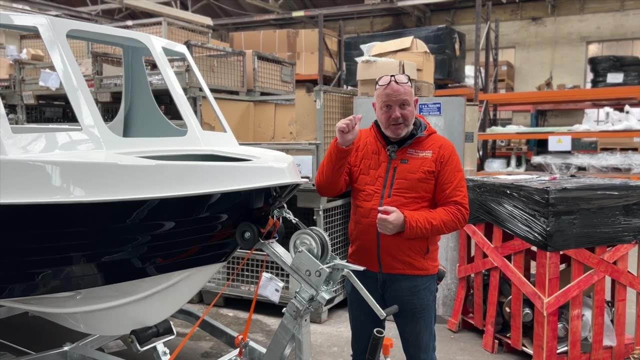 Hi, it's Andy from SBS and people phone up and they want to know what are the key pieces of information they should supply us so we can spec the right trailer for their boat. and it's dead easy. we can do it down to two main pieces of information: the length of your boat and the 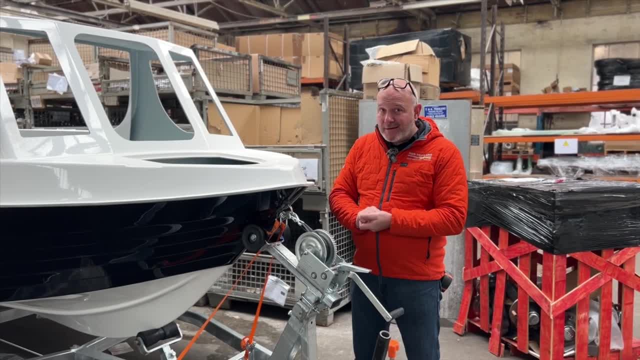 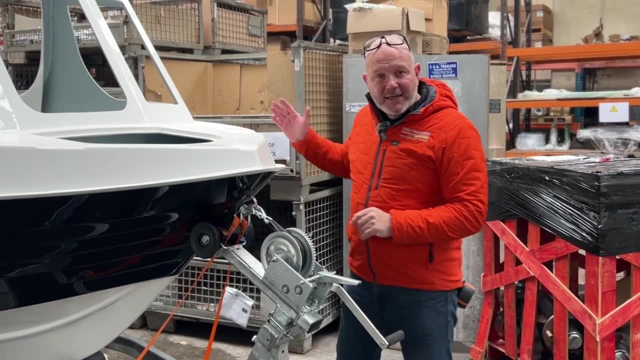 weight of your boat. but within that, it's never easy, is it? because what we really want to know is the supported length of your boat, which is dictated from the bow-eye to the transom, so that won't necessarily be the overall length of the boat. it'll be shorter, so we'll look at what bow-eye 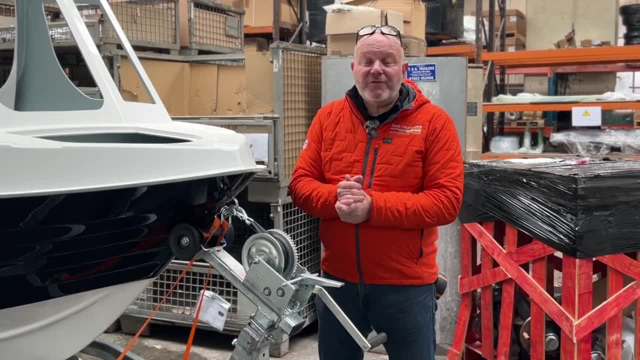 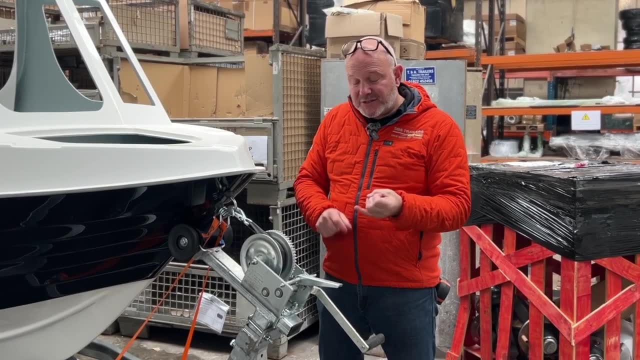 to transom means. and with regards to your weight, the manufacturer, for whatever reason, will notoriously quote the weight a bit light and it might not include the engine as well, so you need to check that out. so we need the weight of the boat combined with the engine and allowance for fuel and 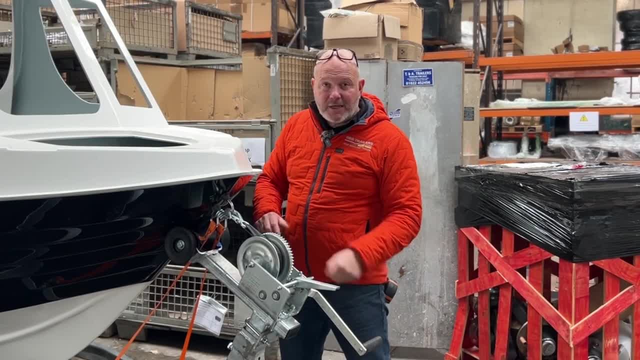 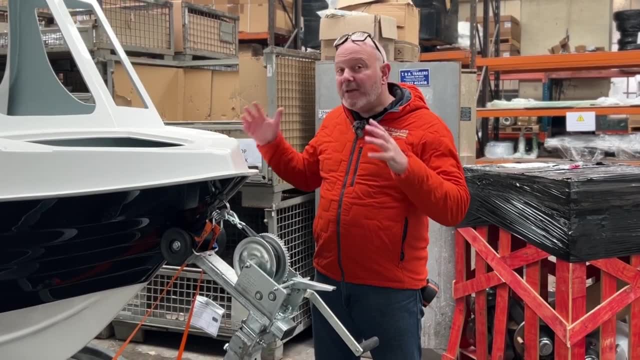 allowance for gear as well. so that suitcase you miss is taken out of the boat and we're going to be looking at the bow-eye to transom and we've got a lot of space in here. so if you're going to travel to the UK and you're going to be on holiday, which is always overweight- you don't get much in. 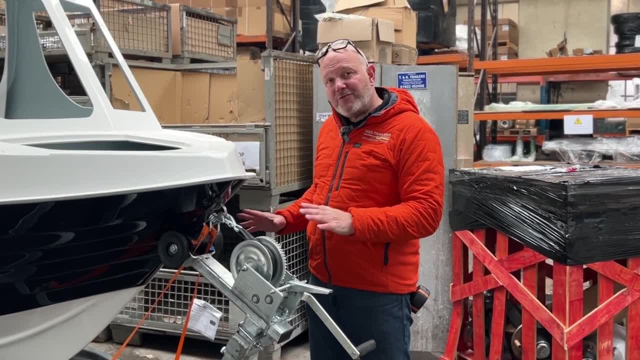 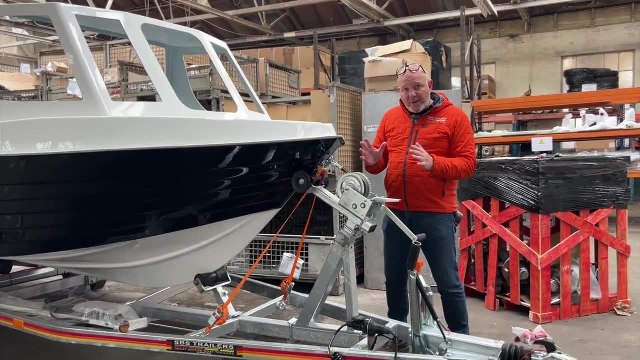 there. so just think about that: when you've got a nice big boat with a lot of space, you can get a lot of gear, which equates to a lot of weight, and you want to give yourself about a 10% headroom just to make sure that the trailer isn't absolutely maxed out from the off, and then you'll be fine. so 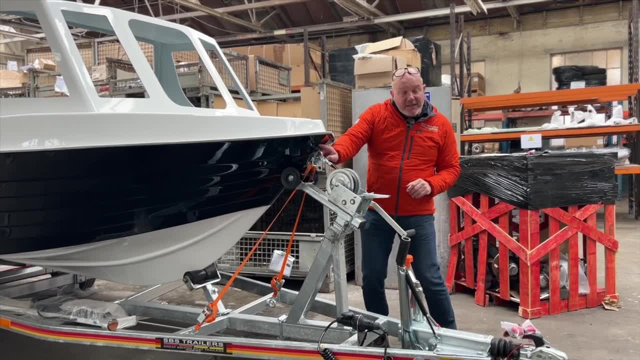 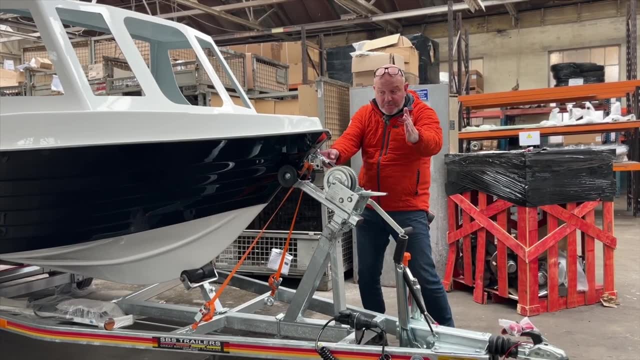 when we look at the bow-eye to transom, you can see in this instance this is a lovely little endeavor that we actually produce here at SBS. this bow-eye is set quite high. imagine if this boat was a rib, so the the overall length of the boat would be that much longer. or indeed, if this bow-eye was. 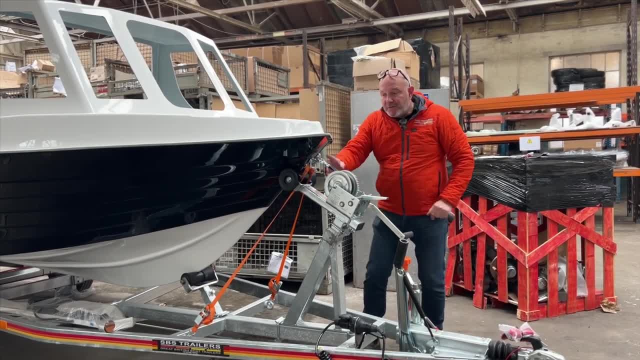 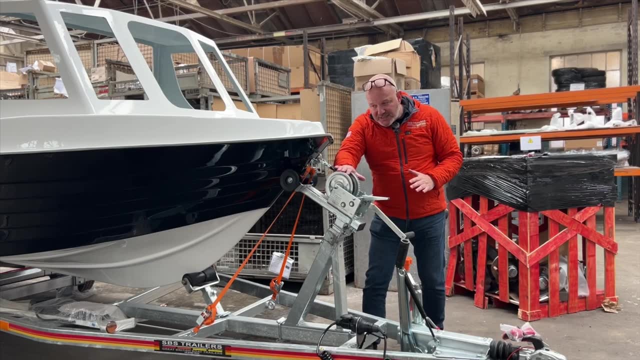 set there. you've now got this bit of overhang, so the bow-eye to transfer will always be shorter than the overall length of the boat. the other thing you want to do is make sure that the winch is in the correct position, so it's pulling the boat on correctly during recovery, and we do a. 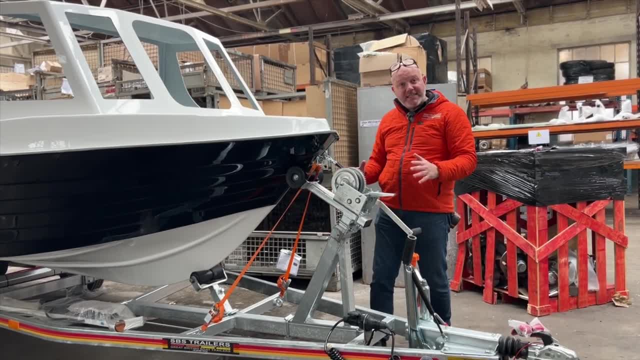 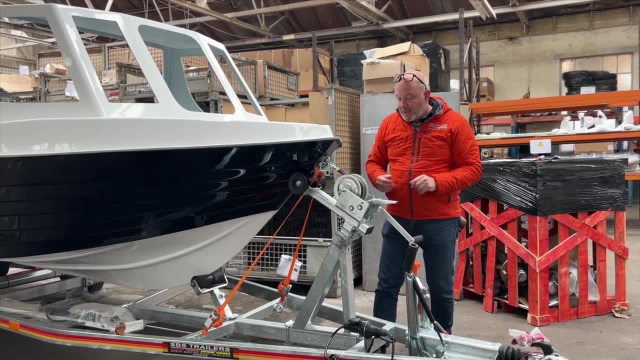 number of different winch post tops and bases to facilitate that, and that'll be part of the almost the consultative discussions that we have during the purchase process. other little things to notice is the bow roller. this is an adjustable roller so you can see, as is the winch post it's held on with.